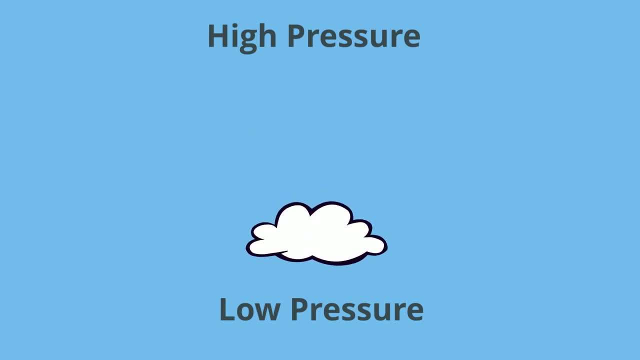 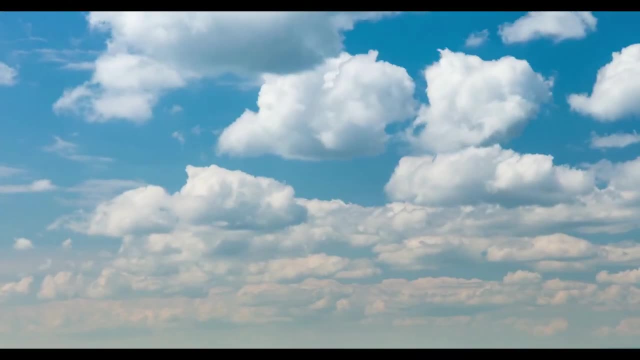 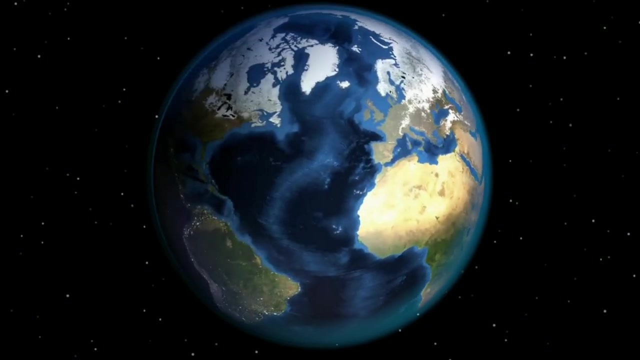 high pressure areas to low pressure areas. Because the earth spins, anything that floats above the earth's surface, such as air, appears to follow a curved pattern of movement. This is called the Coriolis effect. The Coriolis effect heavily impacts the travel pattern of global winds In the northern hemisphere. 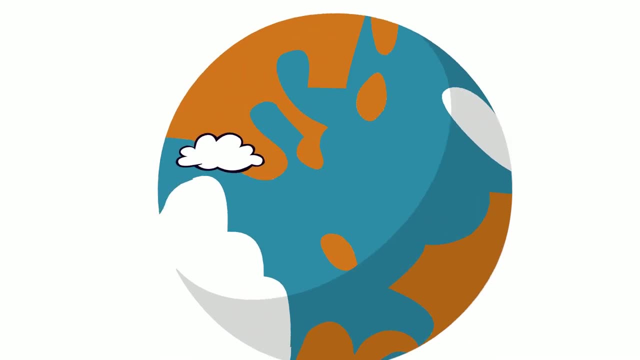 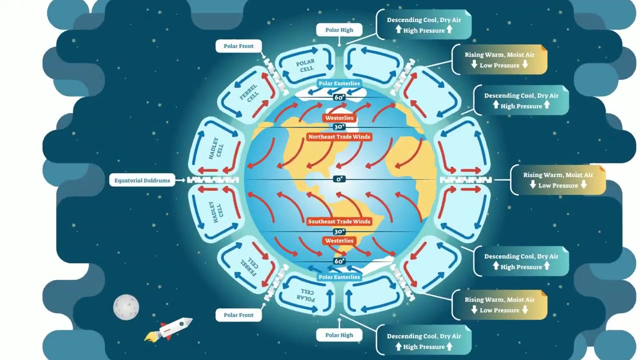 air moving from north to south deflects to the left. From the equator to the poles, air deflects to the right. Now let's put all this together and look at some global winds First. we will label the earth. The direction of the global winds changes every 30 degrees. 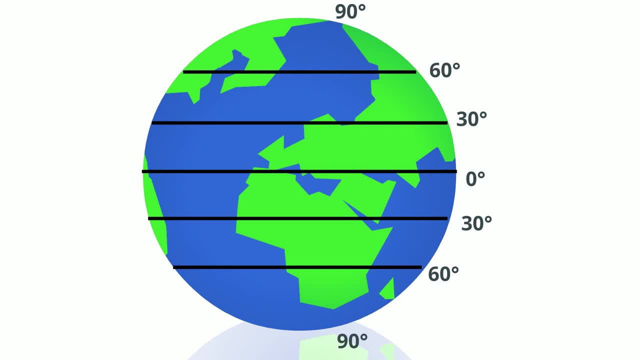 on earth. You can see, I have the earth labeled 90,, 60,, 30, and 0 degrees in the northern and southern hemisphere. At 90 degrees, the air is very cold and dense and creates a high pressure system. At 60 degrees, the air is warmer, resulting in a low pressure system. 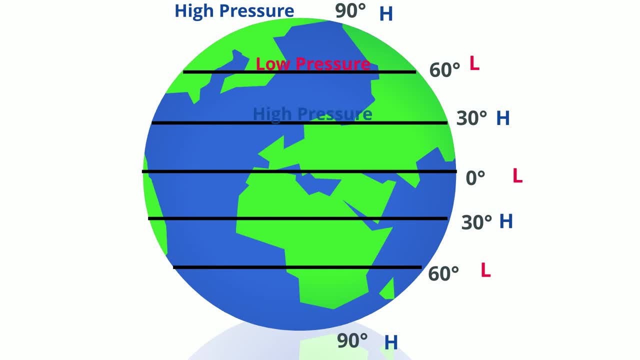 the air is cooler than it is at the equator, creating a high pressure system. It is very hot at the equator and the warm air creates a low pressure area. once again, Notice the alternation between high pressure and low pressure areas: Every 30 degrees witnesses. 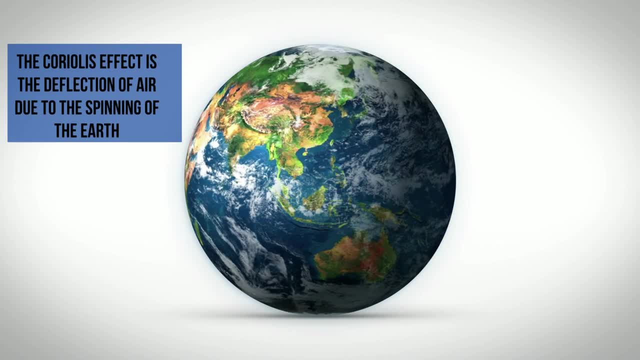 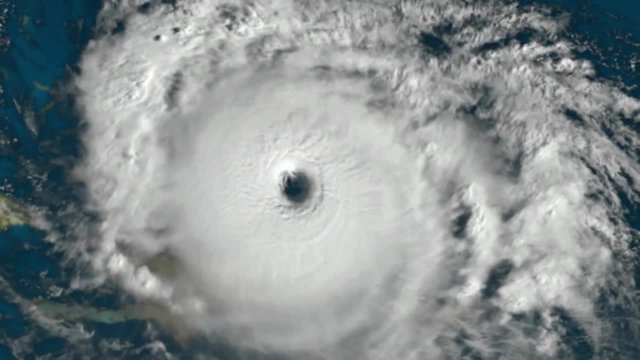 a pressure change. Next, remember that the Coriolis effect heavily impacts airflow. Wind systems will twist clockwise or counterclockwise under the Coriolis effect. In fact, this is what happens with the prevailing winds. There are three main prevailing belts: The prevailing 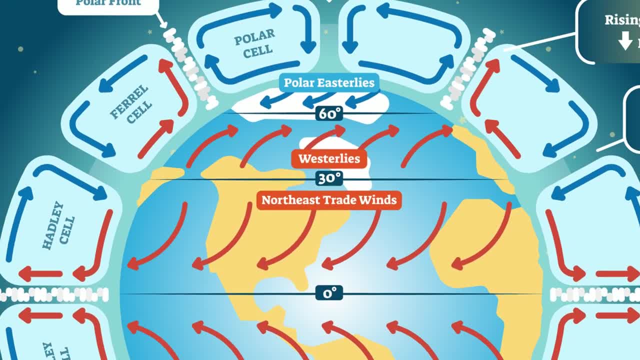 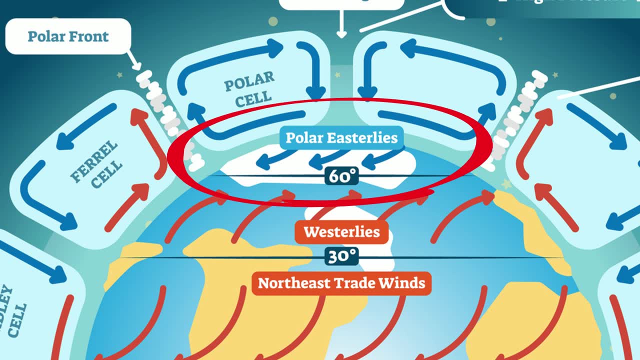 westerlies, the trade winds and the polar easterlies. The polar easterlies are the dominant winds found between 60 degrees of latitude and the poles of the earth. Remember that air likes to move from high pressure areas to low pressure areas, So the wind will start from the poles at 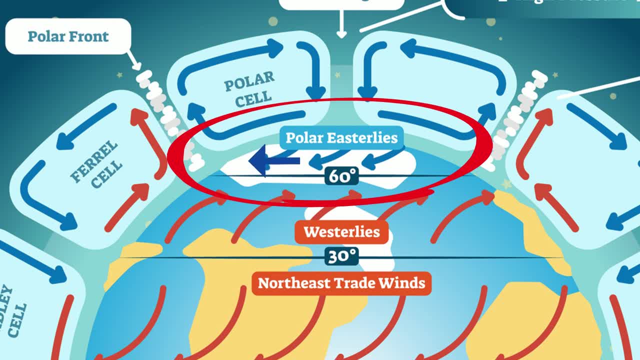 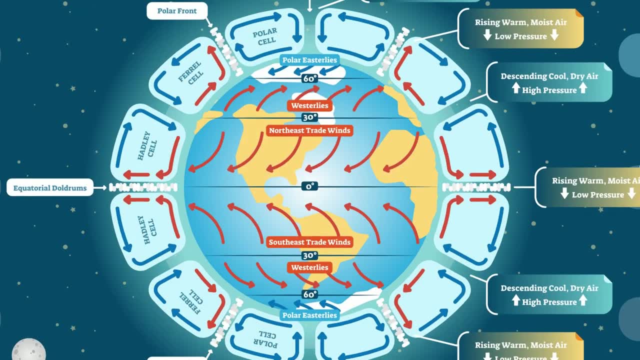 90 degrees areas of high pressure and move down towards 60 degrees where the pressure is low. The prevailing winds will move from high pressure areas to low pressure areas. The prevailing westerlies are the dominant winds found between 30 and 60 degrees of latitude.